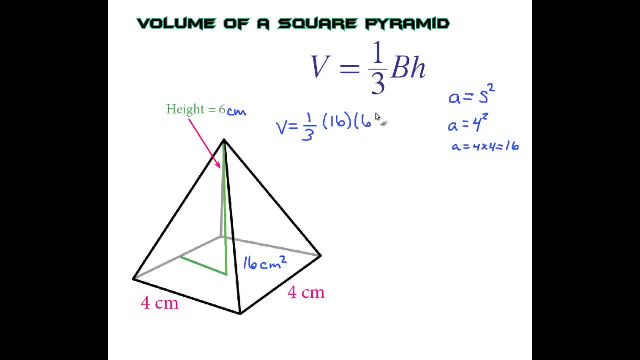 is six centimeters. Let me write that in there. Okay, so now we have everything filled in. Okay, we found out that our base, our flat two-dimensional shape, was a square, And remember that anytime you see a capital B in a volume formula, that's a two-D or a. 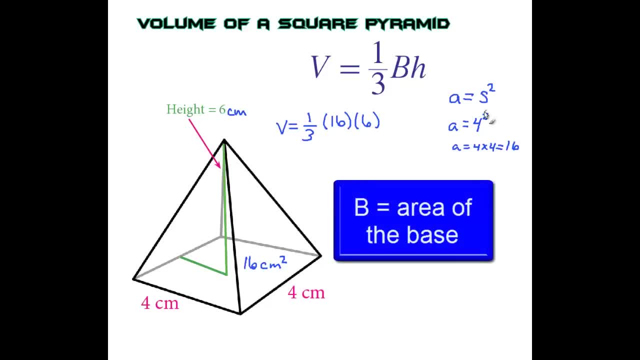 two-dimensional formula for area of the base, In this case a square. We found that it was 16.. So we plug that in here for B, big B, and then we have H, which is equal to 6 for our height. so let's go ahead. 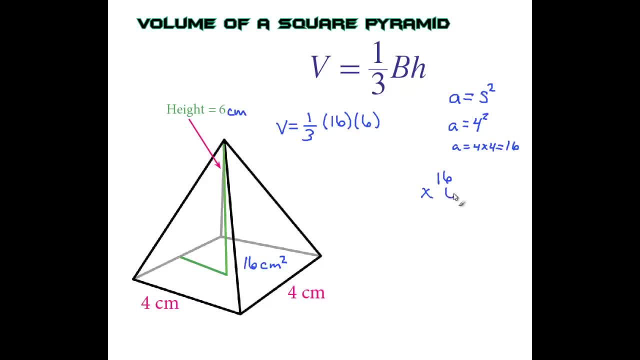 and do some multiplication: 16 times 6 gives us 36 and 9, so we have 96 multiplied by 1. 3rd: now don't get tripped up with this. there's a lot of different ways teachers show this, but I think the easiest way to show this with 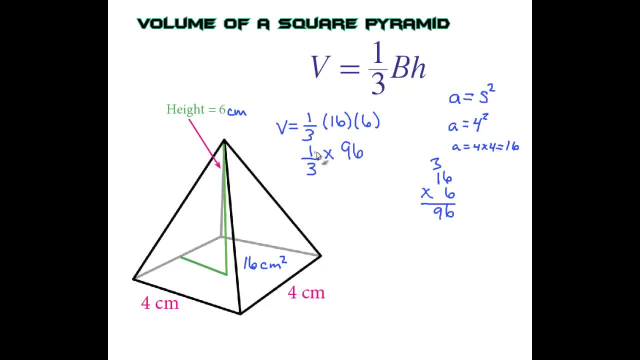 the least amount of steps is just: you're going to multiply the numerator of the fraction to this number here, this whole number here, and then divide by 3. so 1 times 96 gives us 96, and then we're going to divide by 3. okay, go over here. 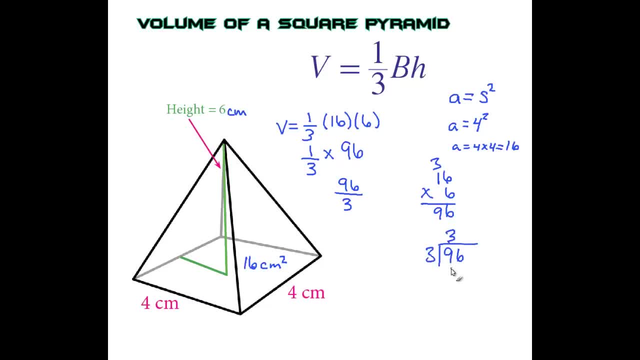 do our little division here and there we go. so the volume of this square pyramid is 32 centimeters cubed. we talk about cubes when we're talking about volume instead of squares for area cubes, because we all love drawing these little cubes here like this, these 3d cubes, okay, so these are. 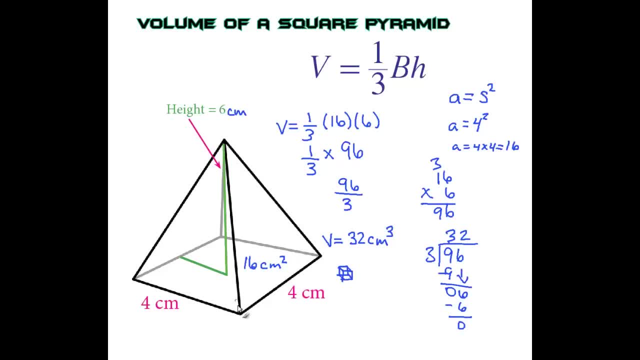 centimeters cubed, we could fit about 32 of them up into this square pyramid here. now, if you struggled with any steps in this problem here on solving for volume of the square pyramid, look at the videos I list at the end and I'm going to list all the supporting skills you need to. 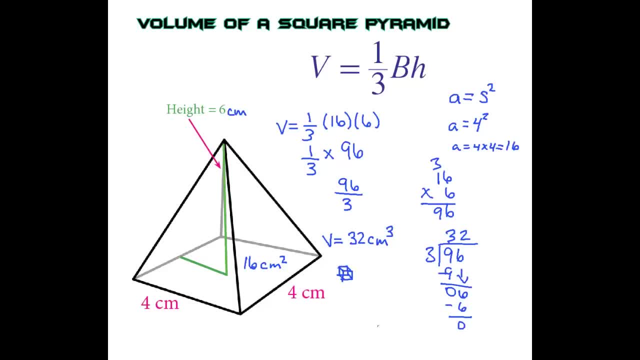 solve for the volume of the square pyramid. thanks for watching. bye, bye.